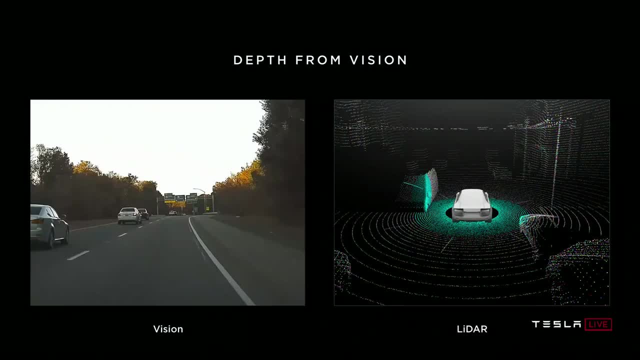 In the car. one is vision cameras just getting pixels and the other is LIDAR that a lot of companies also use, And LIDAR gives you these point measurements of distance around you. Now, one thing I'd like to point out first of all is you all came here, you drove here, many of you, and you used your neural net and vision. 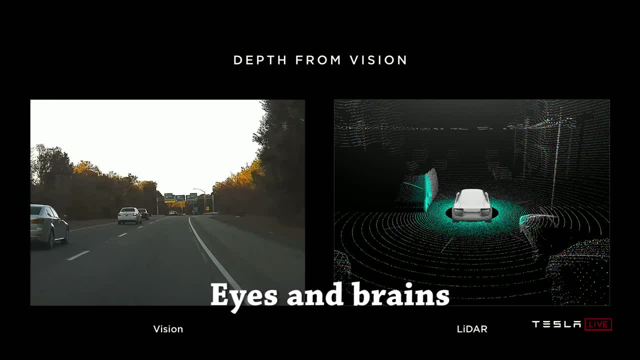 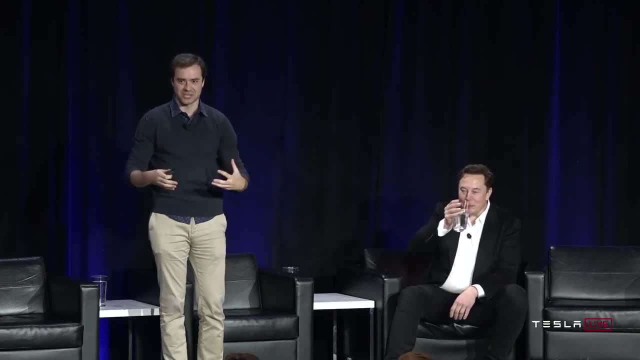 You were not shooting lasers out of your eyes and you still ended up here We might have. So things went well. That's good for everyone. So clearly, the human neural net, The human neural net- derives distance and all the measurements in the 3D understanding of the world just from vision. 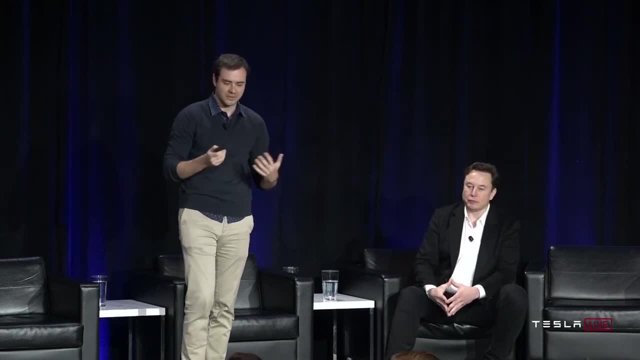 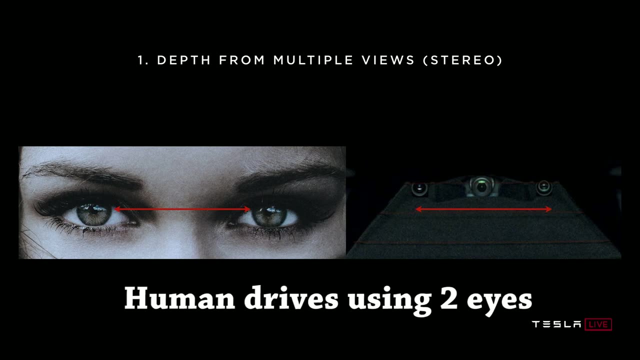 It actually uses multiple cues to do so. I'll just briefly go over some of them just to give you a sense of roughly what's going on inside. As an example, we have two eyes pointed out, So you get two independent measurements at every single time step of the world ahead of you. 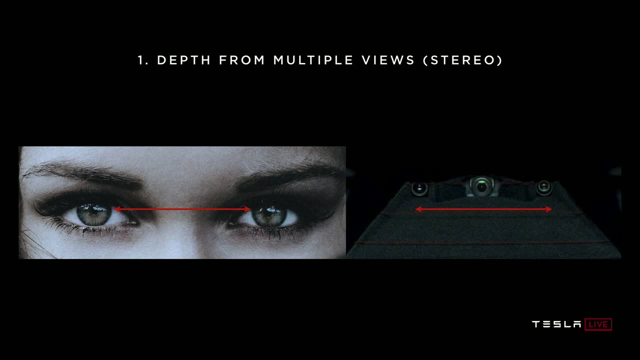 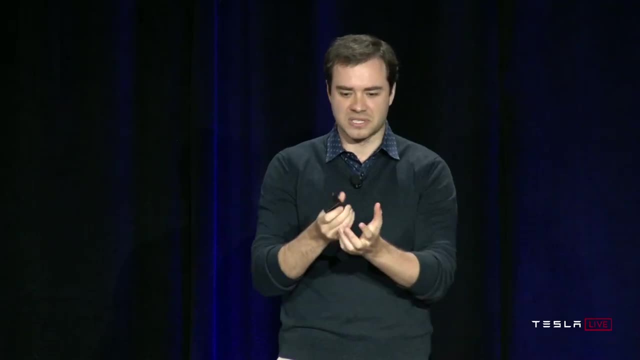 And your brain stitches this information together to arrive at some depth estimation, because you can triangulate any points across those two viewpoints. A lot of animals instead have eyes that are positioned on the sides, So they have vision. They have very little overlap in their visual fields. 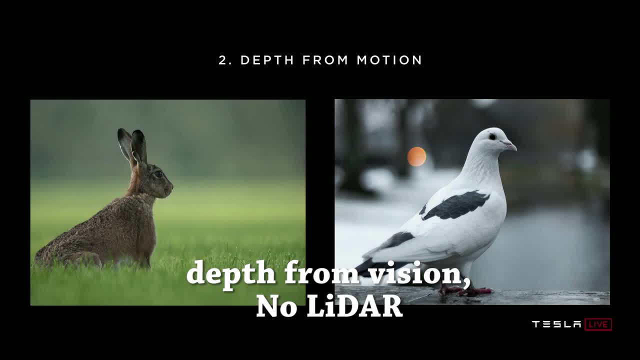 So they will typically use structure from motion And the idea is that they bob their heads And because of the movement they actually get multiple observations of the world And you can triangulate again depths And even with one eye closed and completely motionless you can still have some sense of depth perception. 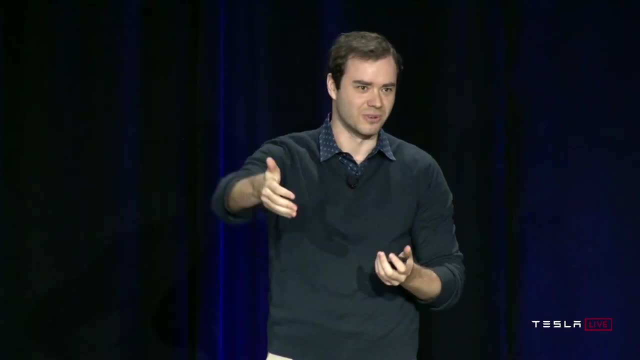 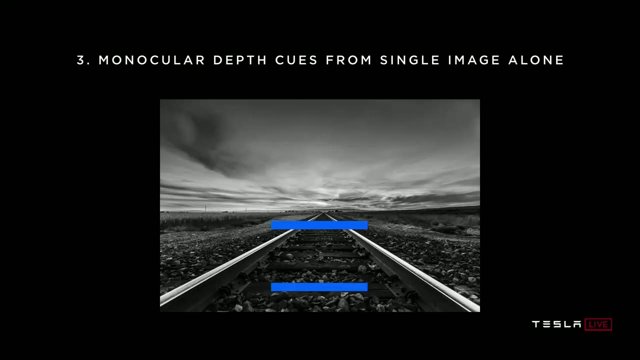 If you did this, I don't think you would notice me coming two meters towards you or 100 meters back, And that's because there are a lot of very strong monocular cues that your brain also takes into account. This is an example of a pretty common visual illusion where you have you know. 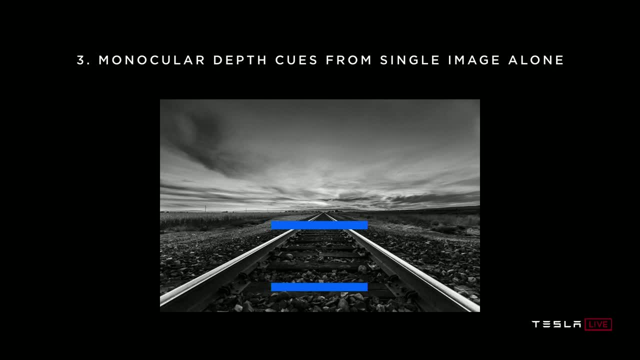 two blue bars are identical, but your brain- the way it stitches up the scene- is it just expects one of them to be larger than the other because of the vanishing lines of this image. So your brain does a lot of this automatically, And neural nets- artificial neural nets- can as well. 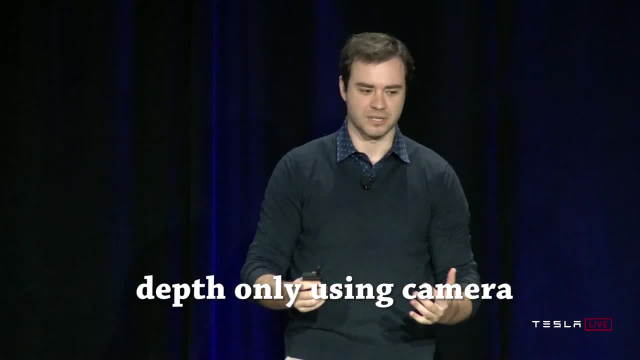 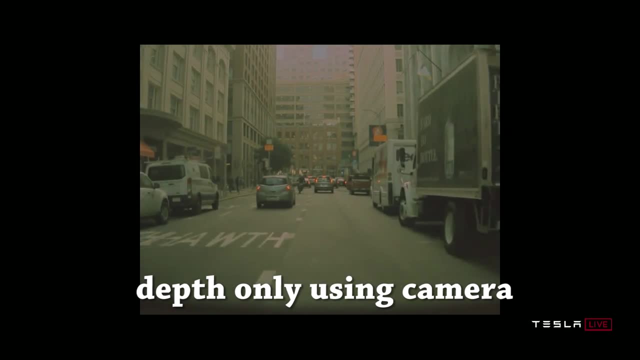 So let me give you three examples of how you can arrive at depth perception from vision alone: A classical approach, and two that rely on neural networks. So here's a video going down- I think this is San Francisco- of a Tesla. So these are our cameras, our sensing. 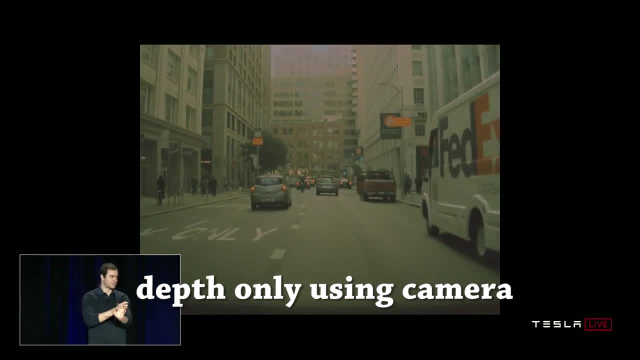 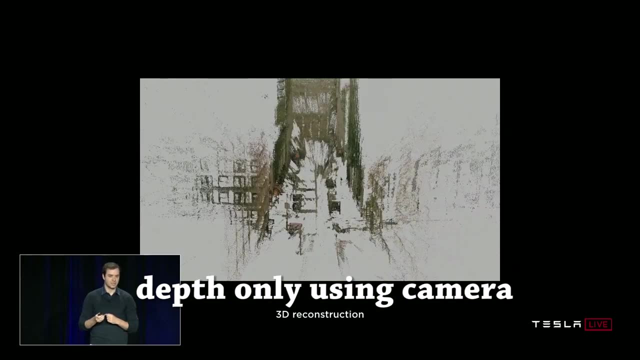 And we're looking at all. I'm only showing the main camera, but all the cameras are turned on- the cameras of the autopilot- And if you just have the six second clip, what you can do is you can stitch up this environment in 3D using multi-view stereo techniques. 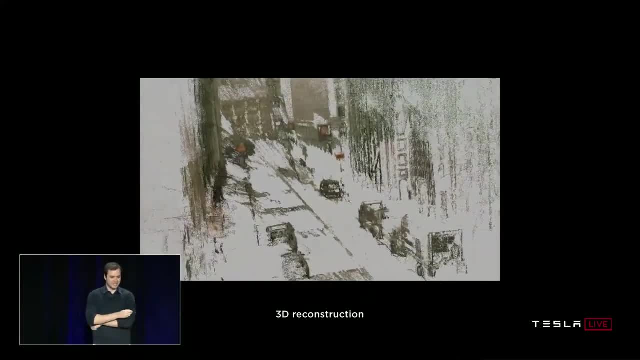 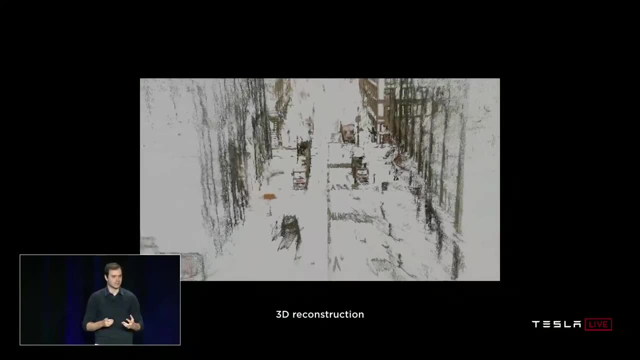 So, oh, there we go. So this is the 3D reconstruction of those six seconds of that car driving through that path, And you can see that this information is purely, is very well recoverable from just videos, And roughly that's through process of triangulation. 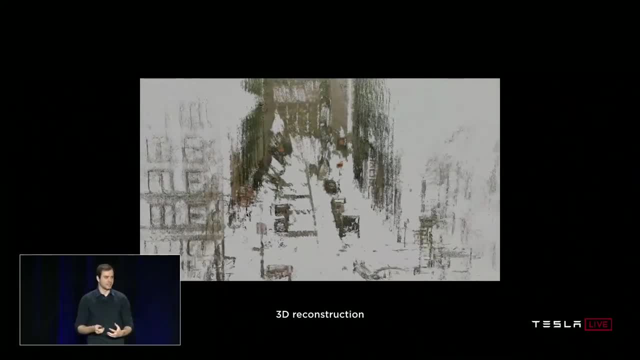 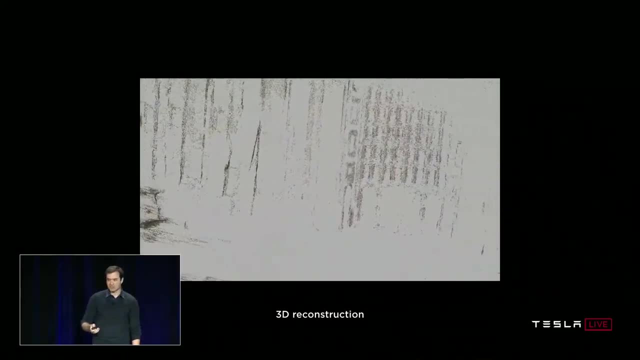 And, as I mentioned, multi-view stereo techniques. So this is the process of triangulation And, as I mentioned, multi-view stereo techniques: stereo, and we've applied similar techniques on a slightly more sparse and approximate also in the car. So it's remarkable. 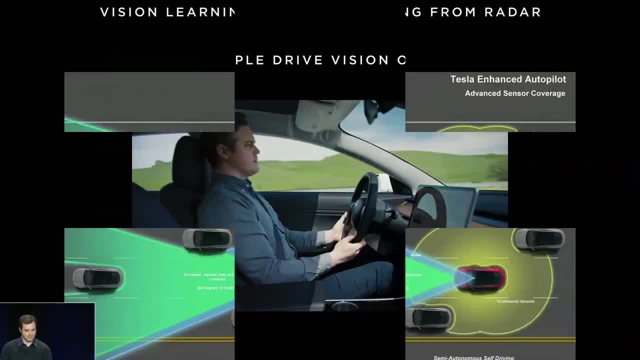 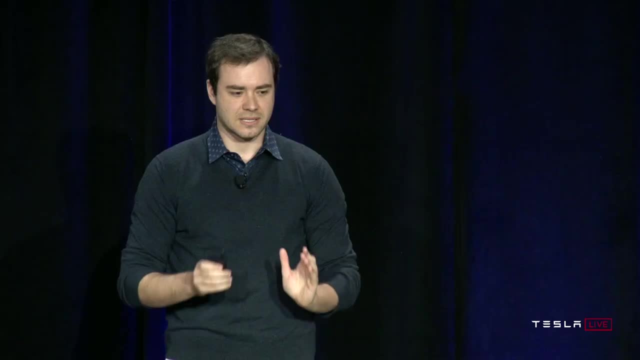 All that information is really there in the sensor and just a matter of extracting it. People drive with vision, only no lasers are involved. This seems to work quite well. The point that I'd like to make is that visual recognition, and very powerful visual recognition- 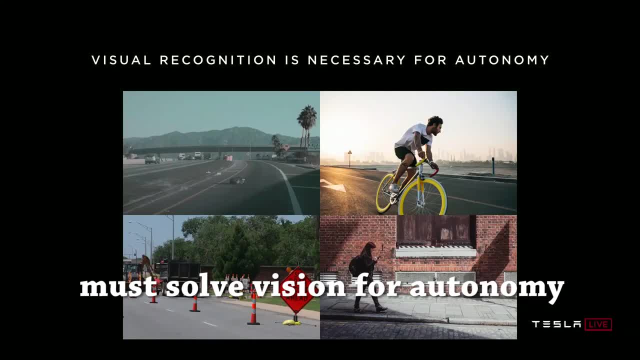 is absolutely necessary for autonomy. It's not a nice to have. You must have neural networks that actually really understand the environment around you And LIDAR points are much less information, rich environment, So vision really understands the full details. Just a few points around are much. there's much less information in those. 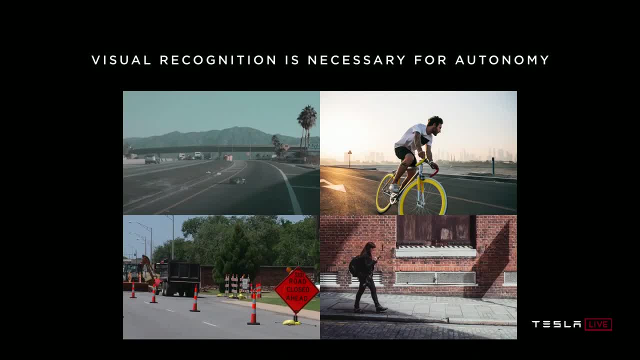 In the construction sites. what do those signs say? How should I behave in this world? The entire infrastructure that we have built up for roads is all designed for human visual consumption. So all the signs, all the traffic lights, everything is designed for vision. 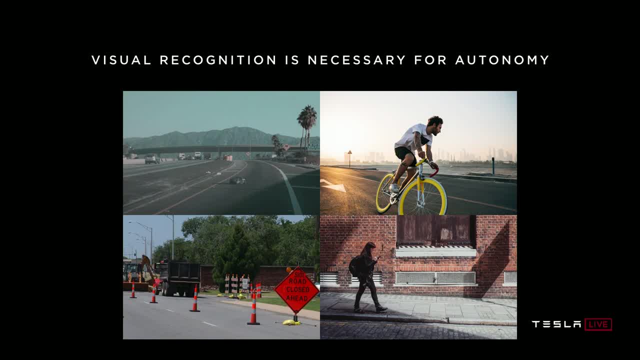 And so that's where all that comes in, All that information is, And so you need that ability. Is that person distracted and on their phone? Are they going to walk into your lane? Those answers to all these questions are only found in vision and are necessary for level. 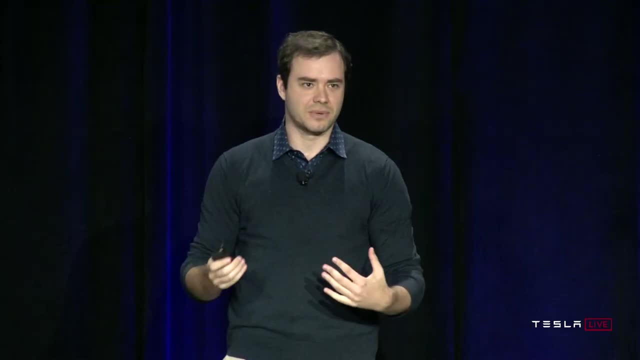 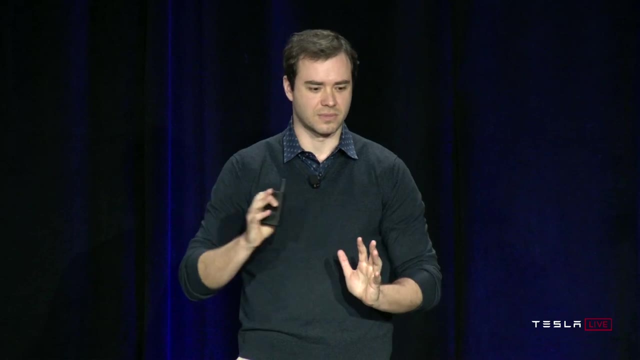 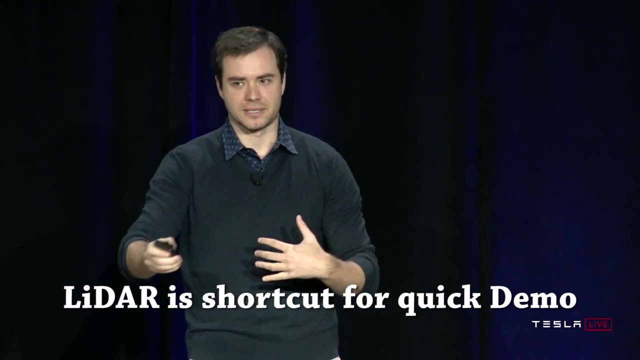 four, level five: autonomy, And that is the capability that we are developing at Tesla And through this is done through combination of large scale neural network training, through data engine and getting that to work over time and using the power of the fleet, And so in this sense LIDAR is really a shortcut. 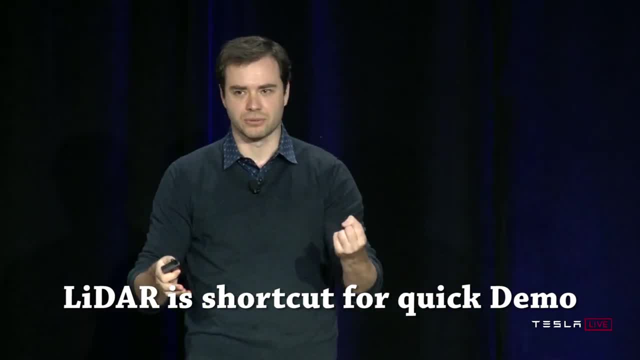 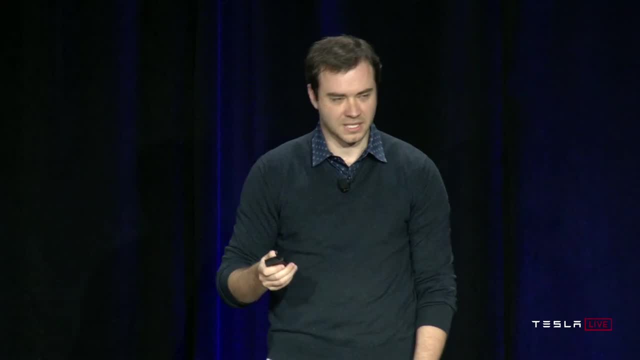 It sidesteps the fundamental problems, the important problem of visual recognition that is necessary for autonomy, And so it gives a full sense of progress and is ultimately- it's ultimately- a crutch. It does give like really fast demos And the autonomous driving you just do with some sensors, LIDAR, radar, et cetera. this